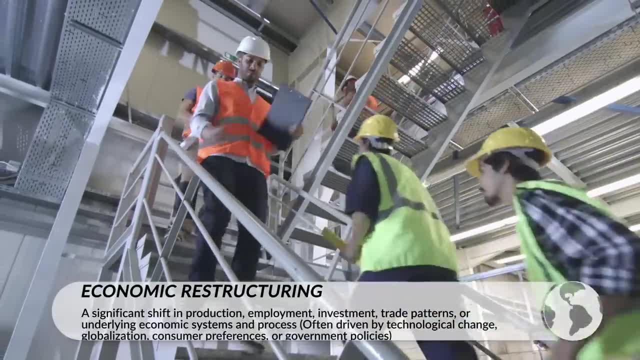 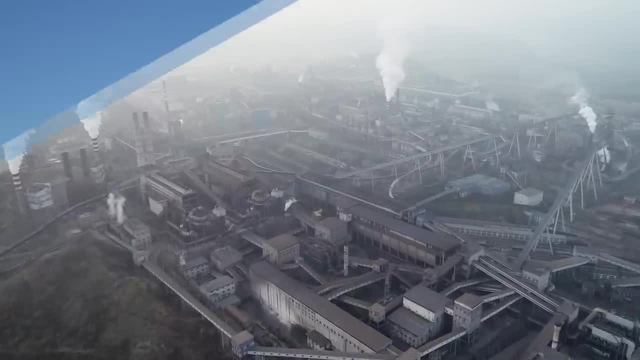 advantage of the new global market. Today, we can see many businesses in core countries move production out of core countries and into semi-periphery and periphery countries. Core countries continue to lose jobs that are part of the secondary sector and have started to lose. 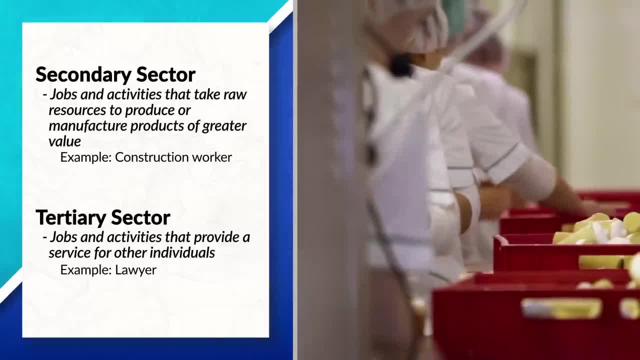 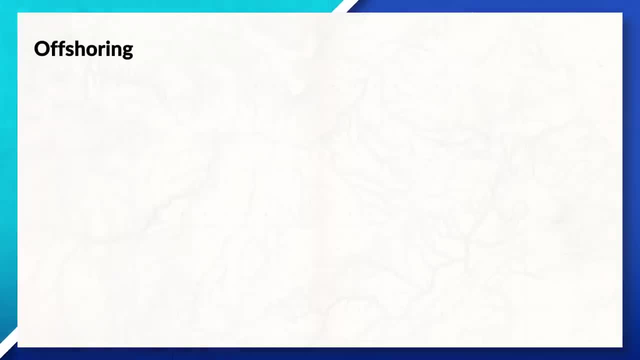 jobs that are in the tertiary sector as well. This is mainly because companies are looking to utilize cheaper labor markets and geographic areas with less regulation. This process of relocating a business's services or processes to a foreign country is known as offshoring. 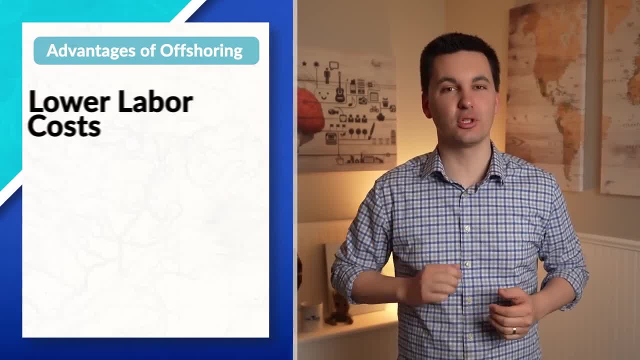 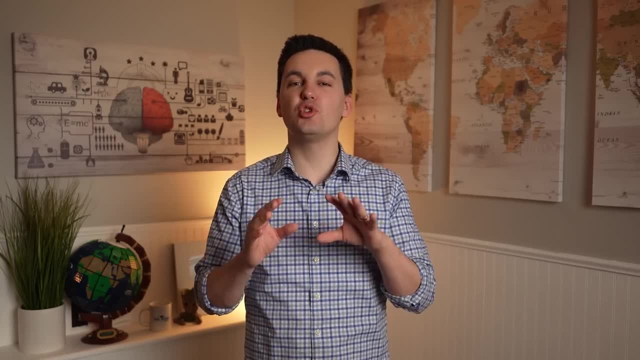 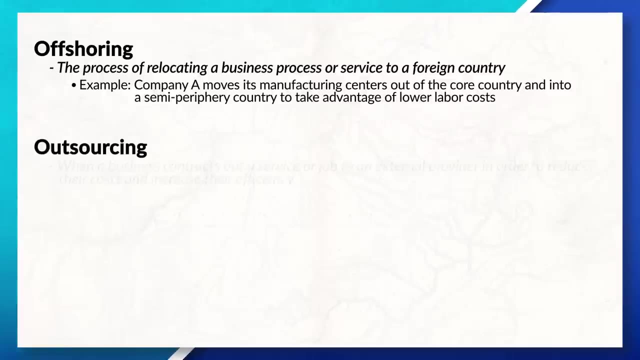 Companies who offshore their production are looking to take advantage of lower labor costs, tax incentives and other favorable economic conditions that exist in a foreign country. Now, another concept you might hear when looking at changes in production is outsourcing, which is similar to offshoring. Outsourcing is when a business contracts out a service or job. 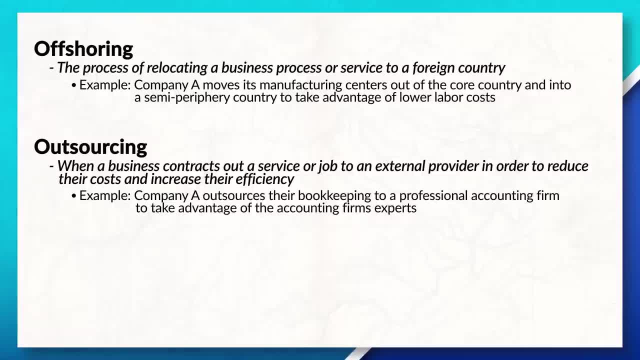 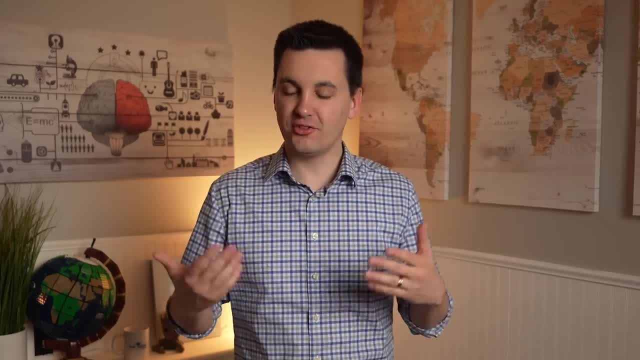 to an external provider in order to reduce their costs and increase their efficiency. Essentially, it is when a company hires another company to do a job or provide a service for them instead of doing it themselves. In addition to outsourcing and offshoring, some companies will also adjust. 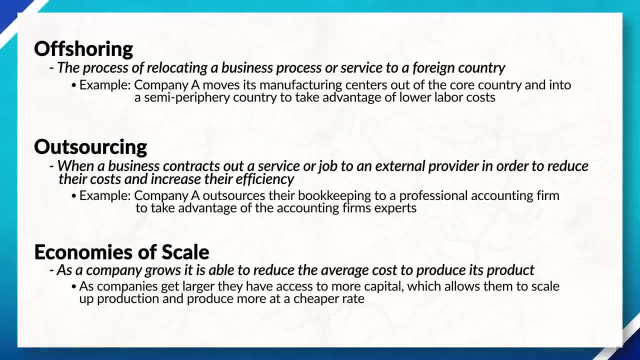 their production based on their size and the economies of scale. So if you're looking to increase your production, you can also increase your production based on your size and the economies of scale. We last talked about this concept in our agriculture unit, where we looked 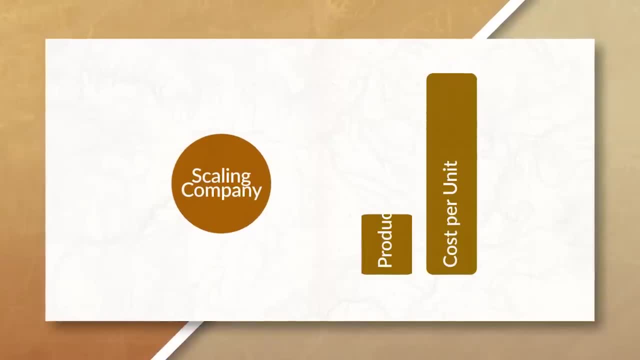 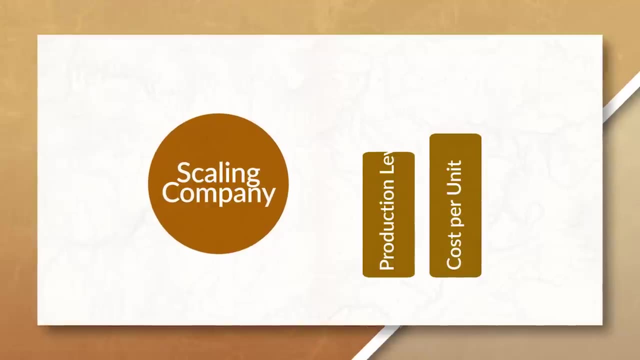 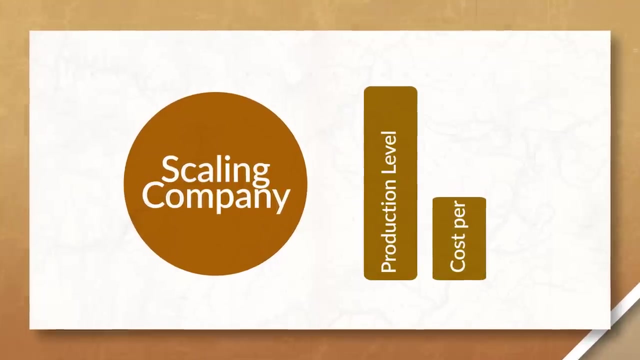 at the spatial organization of agriculture. Companies that are able to achieve economies of scale see a decrease in their cost per unit of production. As companies get larger, they can purchase better machines systems and have more access to capital, which allows them to scale up faster, producing more of a product at a cheaper rate. Large agro businesses. 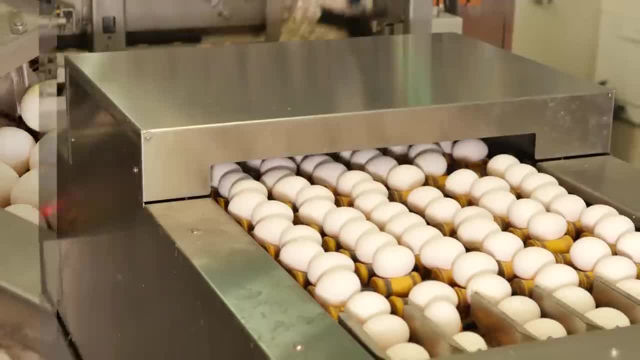 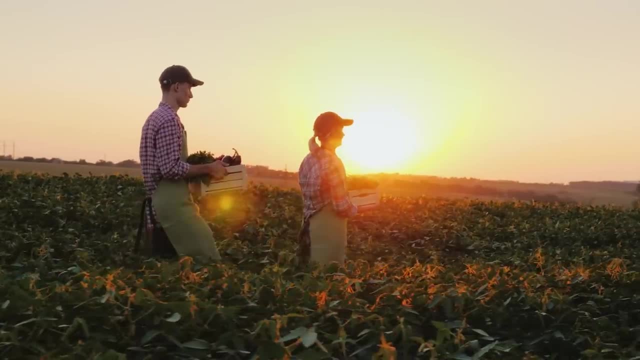 have achieved economies of scale due to advanced machinery that can quickly produce lots of food, which lowers the average cost of each unit produced, making it difficult for family farms to compete in the market with the larger corporate farms. We can also look at the Walt. Disney Company as another company who has achieved economies of scale. Disney owns a variety of different companies that all share their ideas, talents and resources with one another in order to produce high-value content at a lower individual cost. It also has the resources to produce. 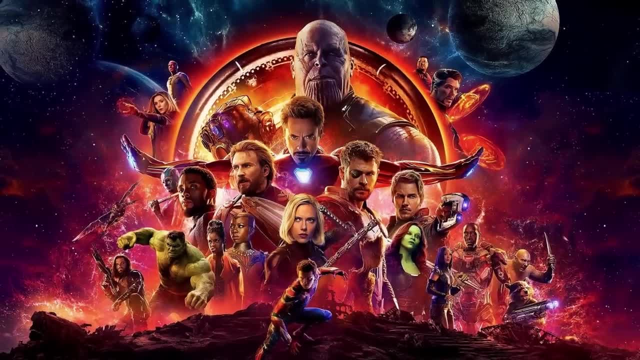 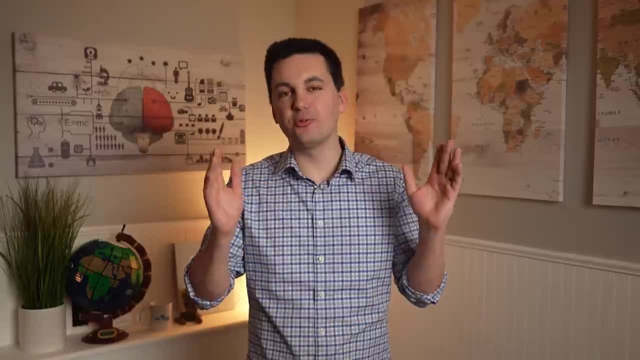 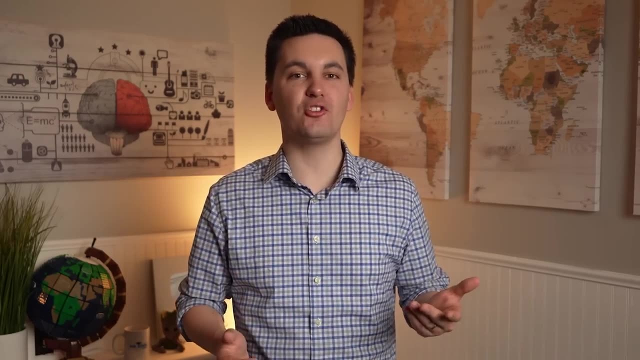 multiple films back-to-back, such as the case with Avengers Inferno, Infinity War and Avengers Endgame, which help save costs by reusing sets, costumes and props, All of which helps Disney reduce their individual costs and increase their overall profits. Now, since we're on the topic of production and minimizing costs, 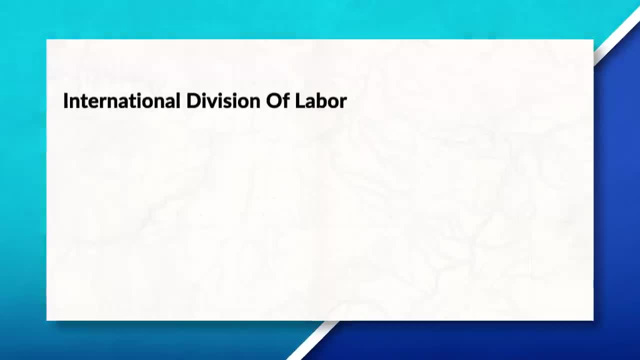 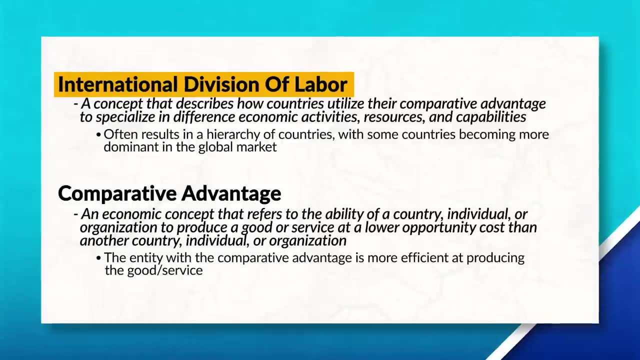 we also have to talk about the International Division of Labor, which is a concept that seeks to illustrate how different countries utilize their comparative advantage to specialize in different economic activities, resources and highlight the country's capabilities. Today, we can see that this global 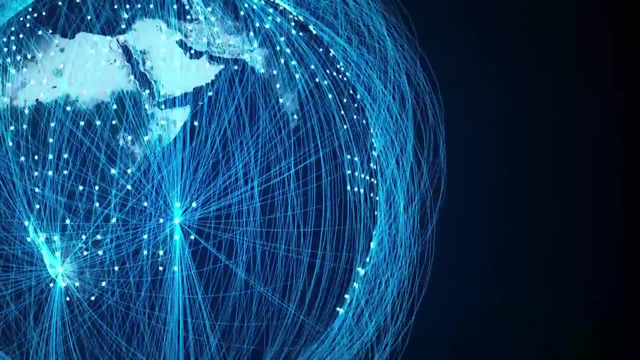 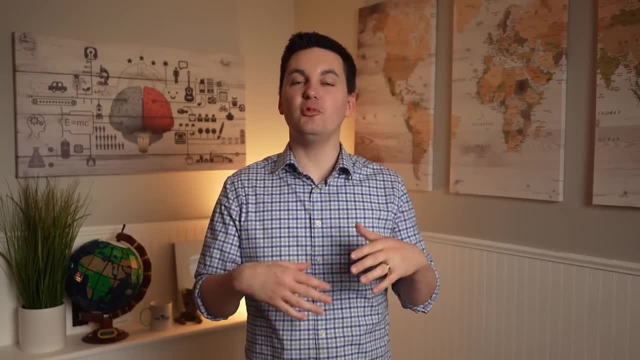 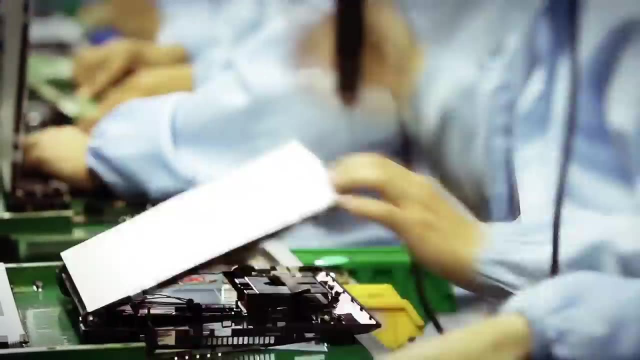 network of trade and production has both positives and negative aspects to it. When countries use the International Division of Labor and focus on their comparative advantage, it allows them to become more efficient at producing specific goods and to trade with other countries to obtain the other goods and services that they are not efficient at. 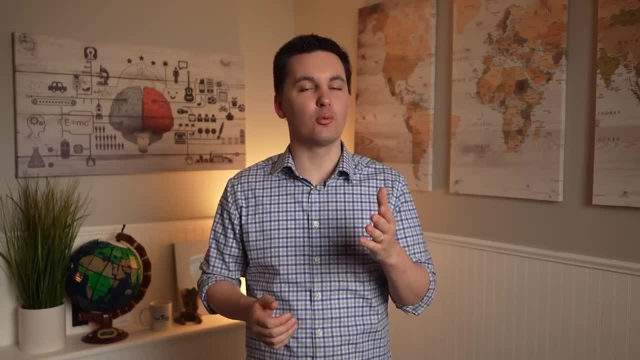 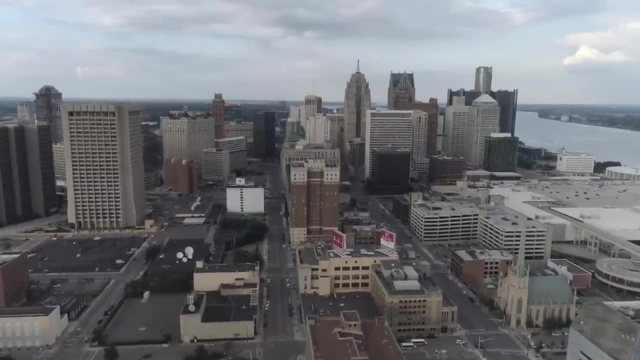 producing. All of which sounds great, but we can also see that there can be some real consequences to this new global market. For example, we can see the negative impact of economic restructuring looking at the city of Detroit. Detroit used to be a thriving industrial city that was known for. being one of the world's top auto manufacturing cities in the world. However, as companies sought to reduce the cost of production, they started to move out of the United States and into less economically developed countries, causing Detroit to experience deindustrialization. 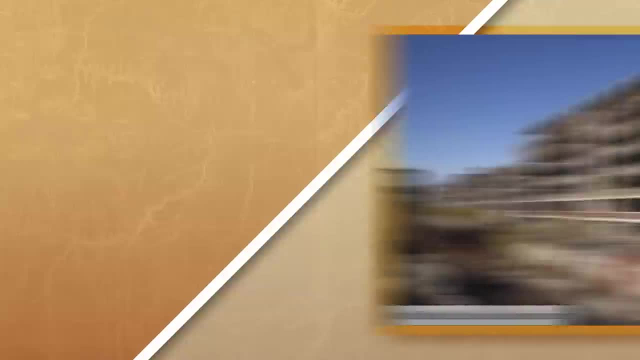 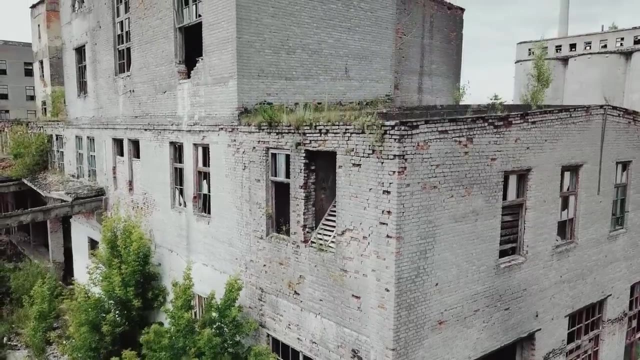 as economic restructuring devastated the city's economy. The loss of the auto industry resulted in the loss of the city's main economic driver. As jobs left the city, so did many of the people, all of which increased the amount of vacant buildings on the market Over time. 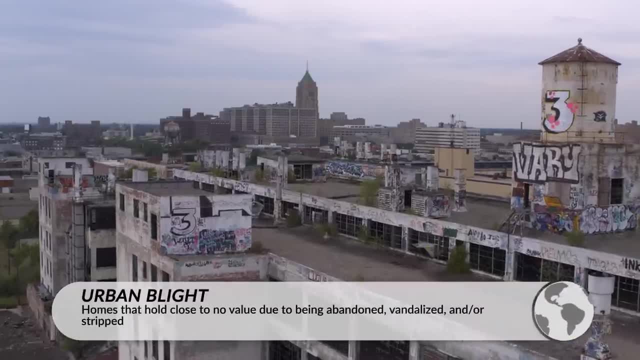 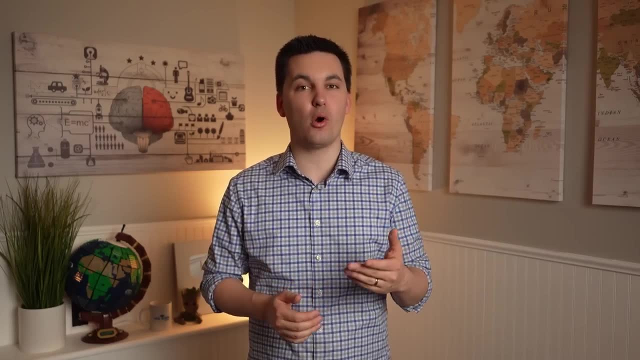 we started to see increased rates of urban blight as homes and buildings were stripped of all value, vandalized and left for decay. Now, as countries continue to participate more and more in the global economy, they will continue to see economic restructuring occur. Core countries will continue. 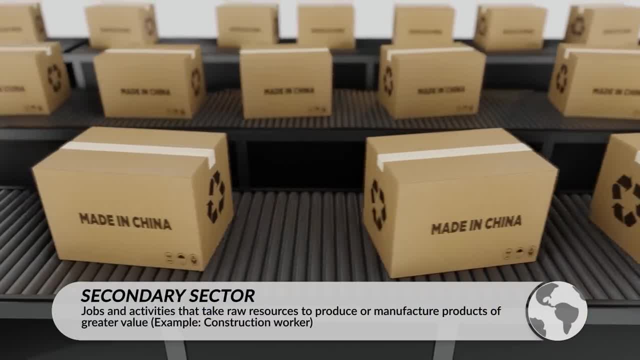 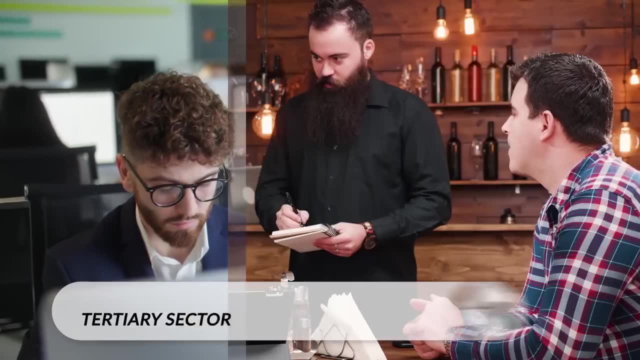 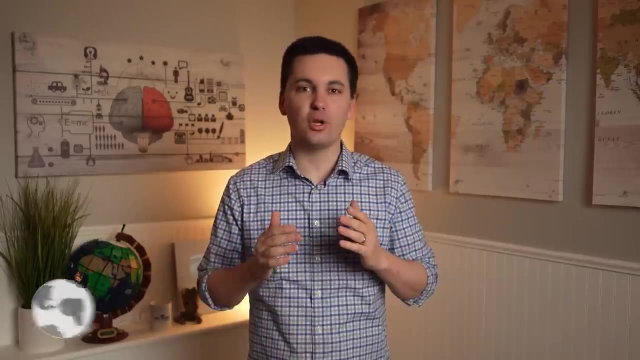 to see more of their secondary sector relocate out of the country and into the developed world, as their economy shifts away from manufacturing and continues to transition into more of a service-based economy, with the majority of the jobs being located in the tertiary sector. Today we can see semi-perforated and perforated countries seeking to increase. 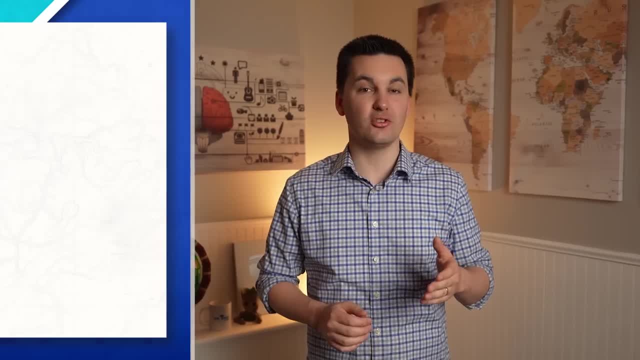 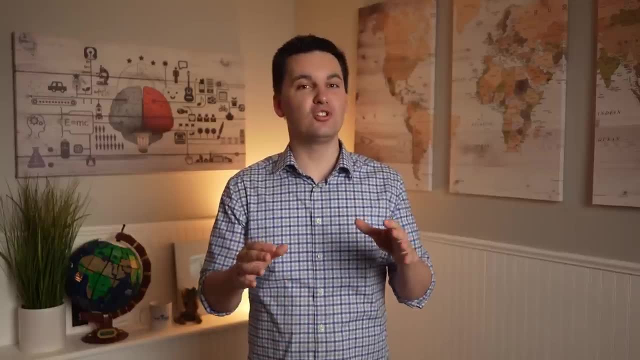 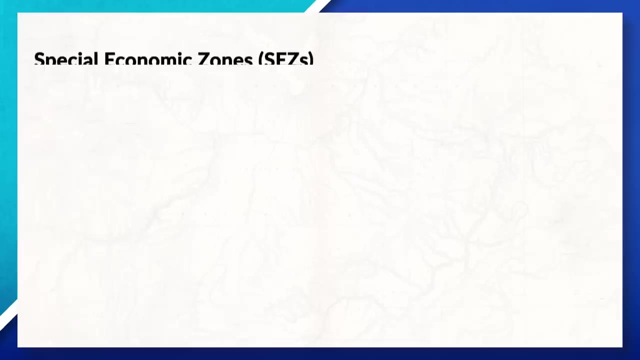 economic investment from multinational corporations and core countries by creating special economic zones, free trade zones and export processing zones, all of which lead to more globalization and economic restructuring, both for core countries and semi-perforated and perforated countries. Special economic zones are areas that seek to provide different incentives. 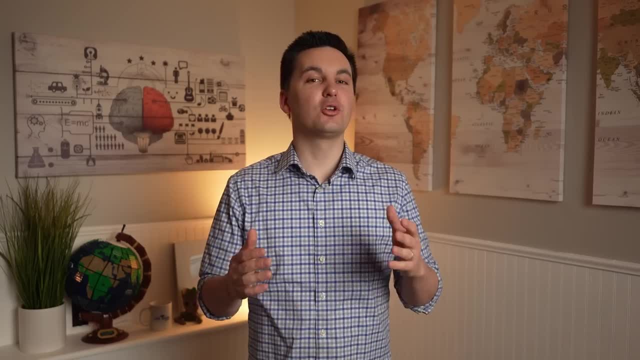 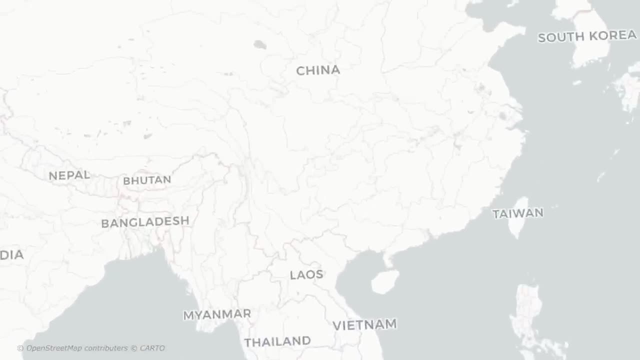 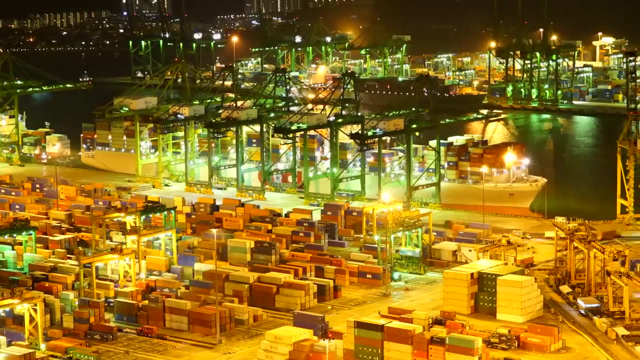 and benefits to businesses who operate in the area. This could include tax breaks, less regulations or access to different services and infrastructure. The goal here is to attract foreign investment from multinational corporations and core countries to help promote economic development in the area. Companies that locate in special economic zones are given preferential. 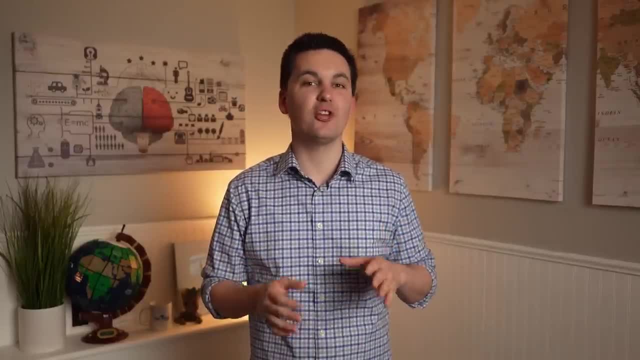 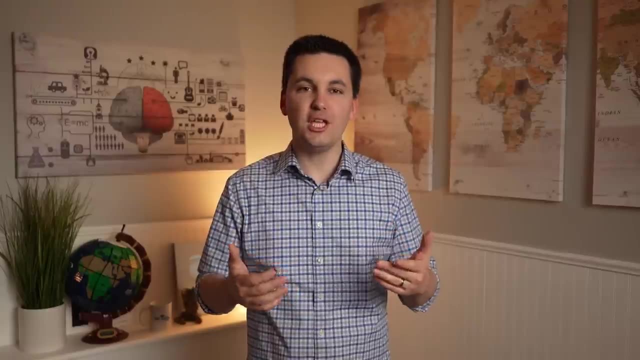 treatment and do not have to follow the same laws and regulations as the rest of the country. Now, both free trade zones and export processing zones are a form of a special economic zone. However, they each focus on a specific goal. Free trade zones are areas within: 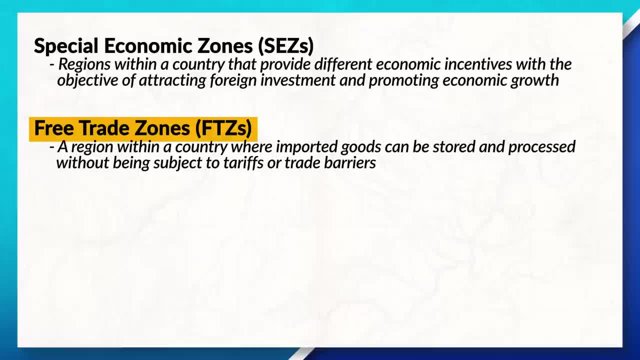 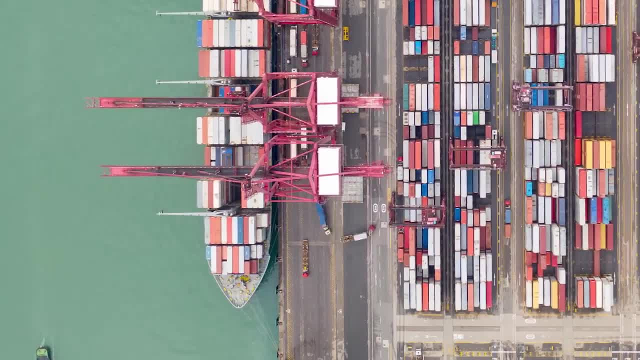 a country that also seek to promote global trade. These areas allow for companies to import and export different products without having to pay tariffs or custom duties. These zones are often centered around a port or infrastructure that allows for the movement of goods in and out of an. 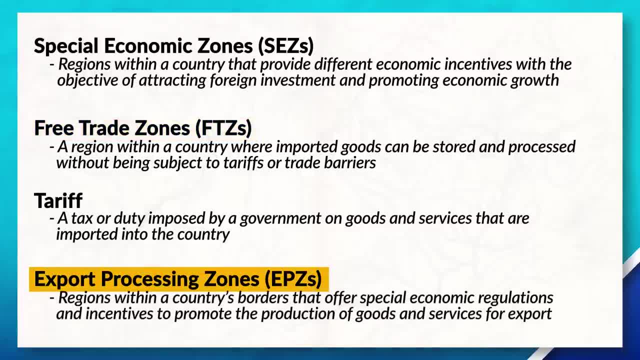 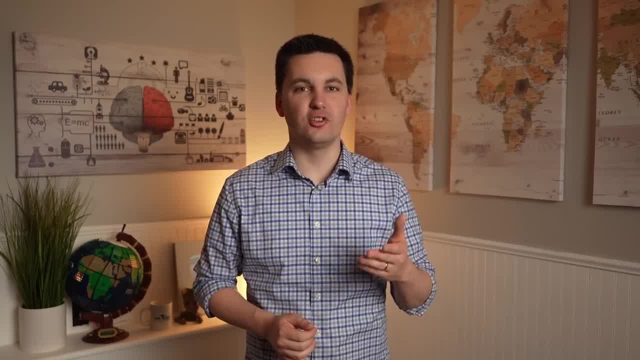 area. Lastly, export processing zones are areas that have the goal of prioritizing the exportation of different goods out of the area. These have the primary focus on manufacturing goods in the area and then exporting those goods to a different country. An example of an export processing zone: 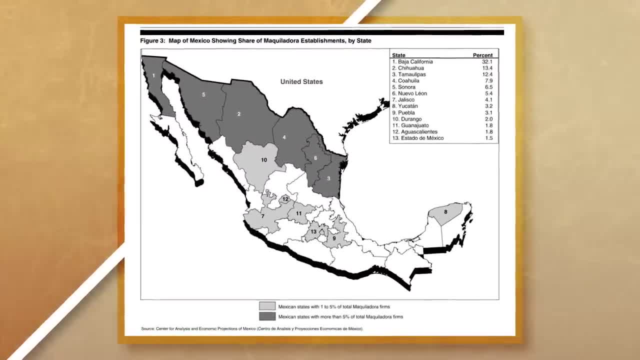 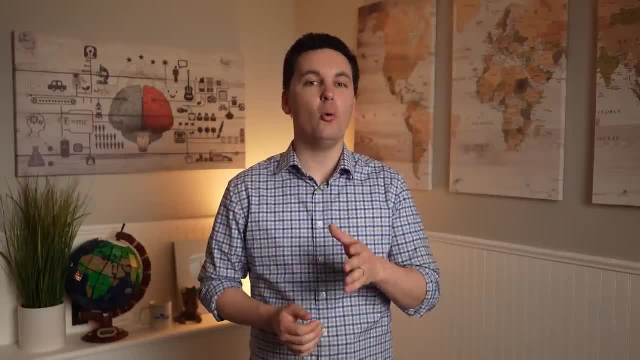 would be Maquiladora, which are manufacturing plants that are located in Mexico along the United States-Mexico border. This export processing zone was created by the Mexican government with the hopes of attracting foreign investment from the United States to produce products in Mexico. This 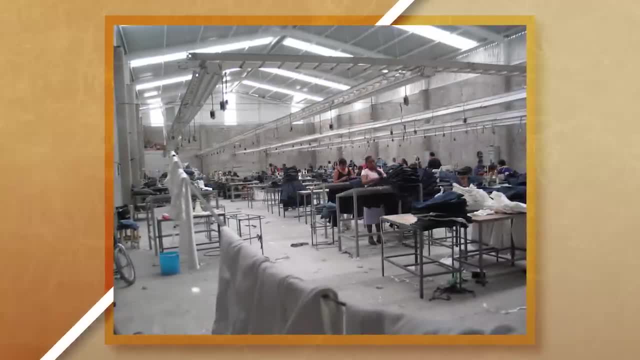 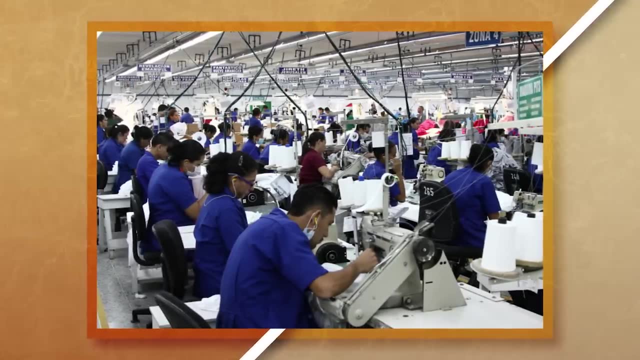 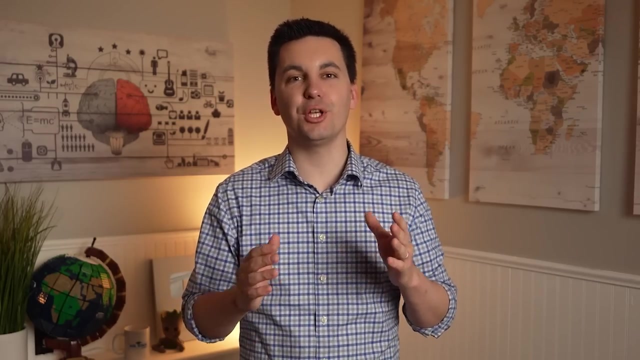 increased local jobs in the area and also the amount of exports from Mexico to the United States. Companies that produce products in a Maquiladora are able to utilize the cheaper labor force in Mexico, which allows companies to reduce their overall costs of production. All of these policies reshape the global international market of labor as they allow. 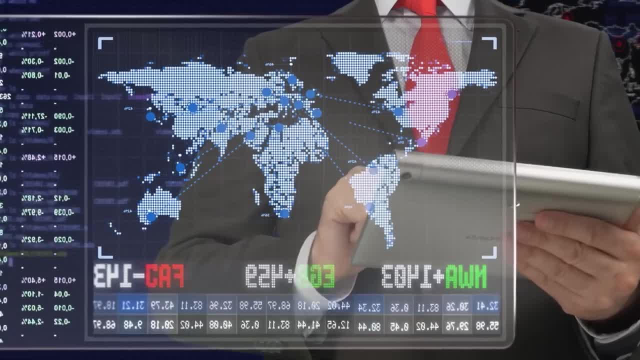 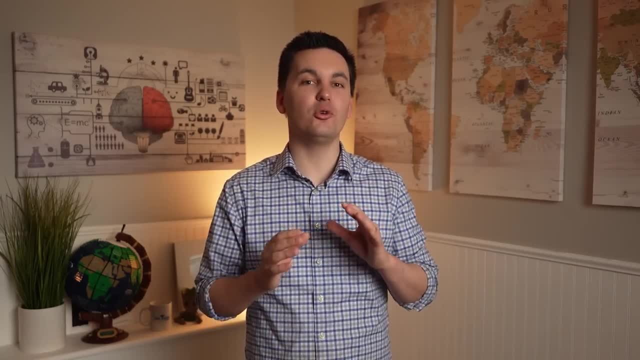 for countries to take advantage of their comparative advantage, specialize more and trade more easily with countries around the world. Before we delve deeper into the production of different products, I want to also talk about the multiplier effect. The multiplier effect looks at how an original investment 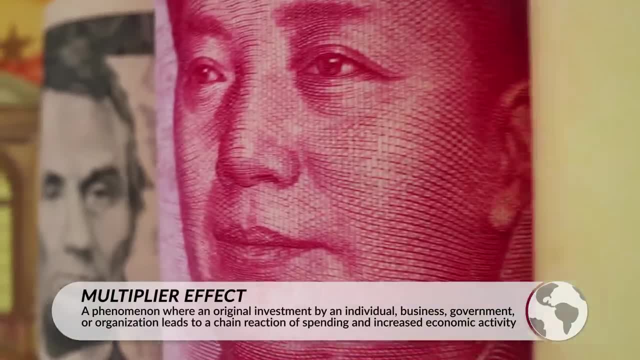 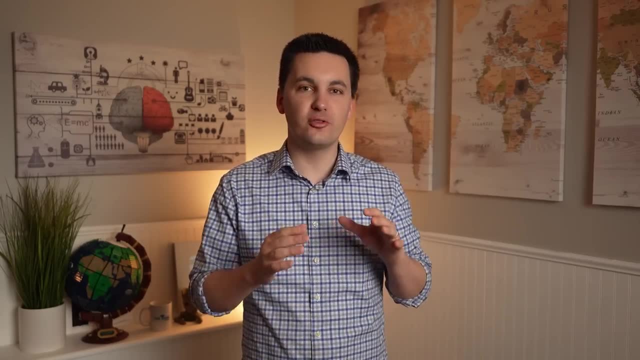 into an economy can create a ripple effect and end up creating a larger impact than the original amount spent. Essentially, when a person, organization or government spends money, it creates a chain reaction of additional spending. Think of it this way. Let's say: 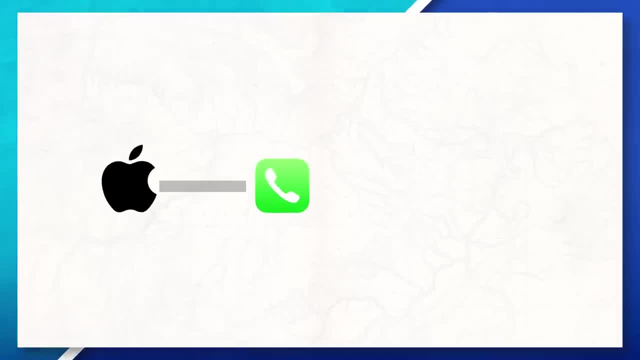 Apple decided to offshore some of their call centers and they open a new call center up in India. This center will have to be built, so Apple will have to pay for a construction company to build the facility and pay for all the different resources needed for the building. Apple will then 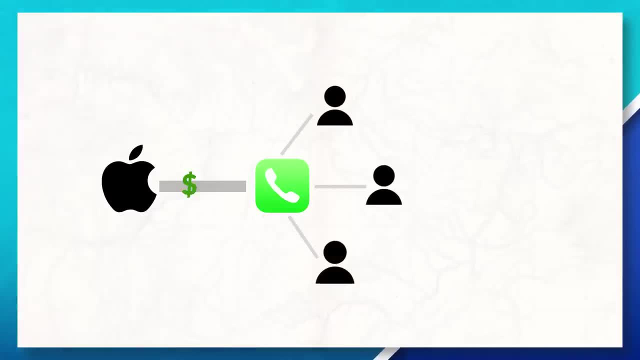 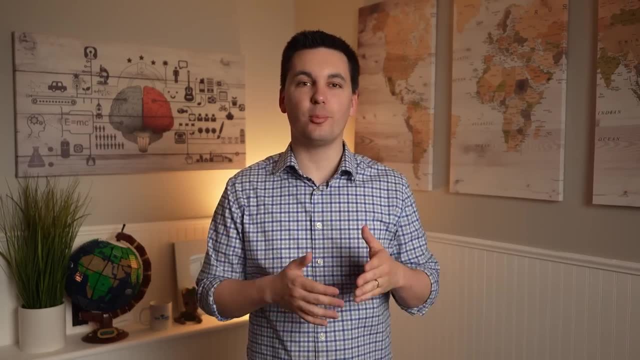 have to staff the building, where they will pay people every day to answer calls and provide support for the company. In this example, the original investment made by Apple is the building of the call center and the workers they are paying to run the center, But where the multiplier effect. 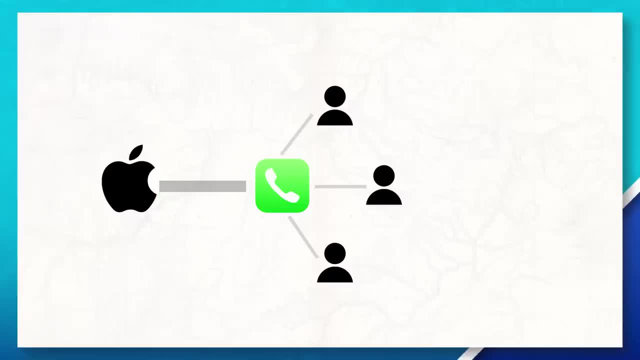 occurs is after the original investment. All of these workers that have been paid by Apple now have more money to either save or more money to purchase other products and items, If the workers from the call center go and spend the money they earn from Apple. they end up supporting other businesses, which increases the amount of economic activity and employment in the area. As those other businesses get more revenue, it allows them to hire more workers, produce more products and support the economy. The people who work at these other businesses then have more access to money and will most 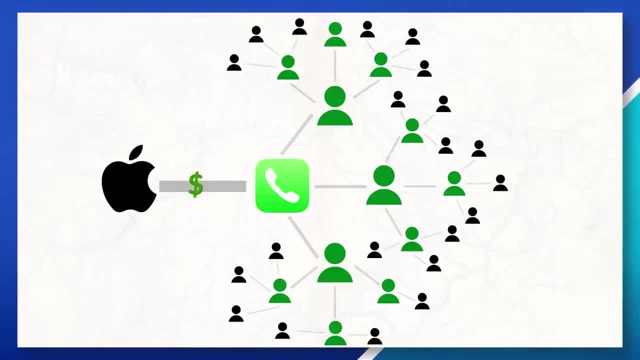 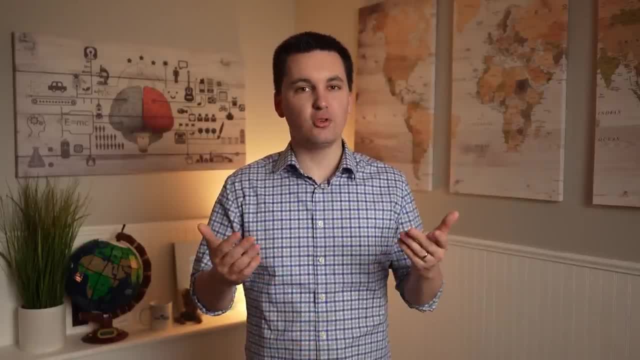 likely go out and spend it, which ends up supporting other businesses and people. So we can see how this original investment from Apple created a chain reaction of additional spending, which ends up increasing the economic activity in the area. Now, today, it is not just globalization that is changing how and where companies and 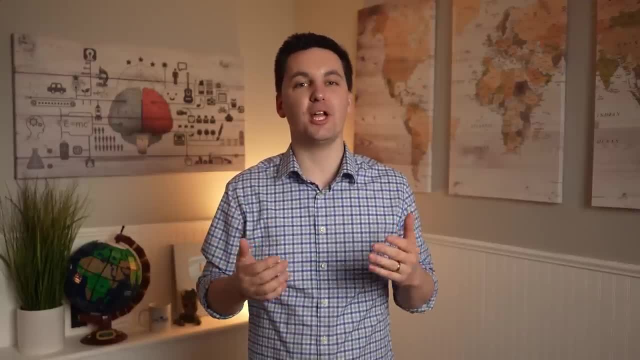 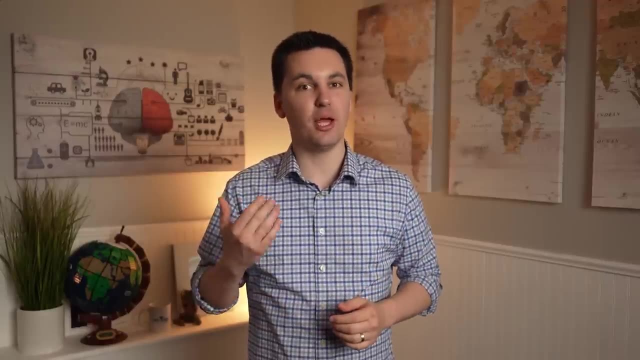 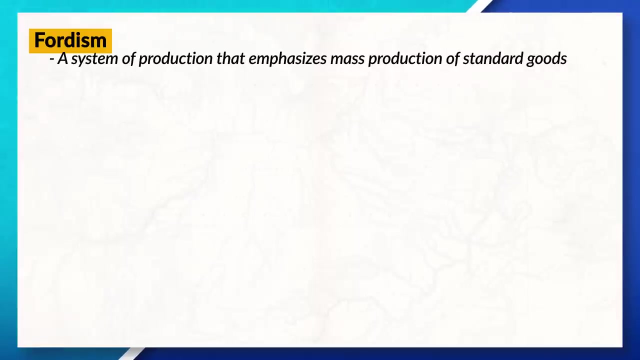 companies produce their products. We can also see how the contemporary economic landscape is changing, as countries continue to shift from Fordist methods of production to post-Fordist methods of production. Fordism emphasizes mass production of standard goods in a large factory that uses assembly lines for production. This production method has a set. 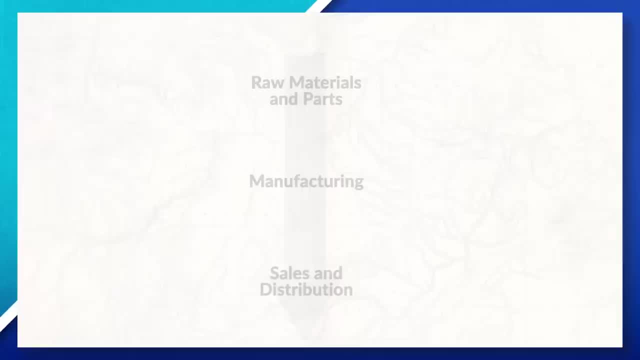 division of labor, with each worker performing specific tasks. Decisions and production under Fordism are centralized, with a greater focus being put on standardization. Post-Fordism, on the other hand, emphasizes more flexible production methods which are able to adjust to the daily changes of the market. This production method also has workers be trained in multiple 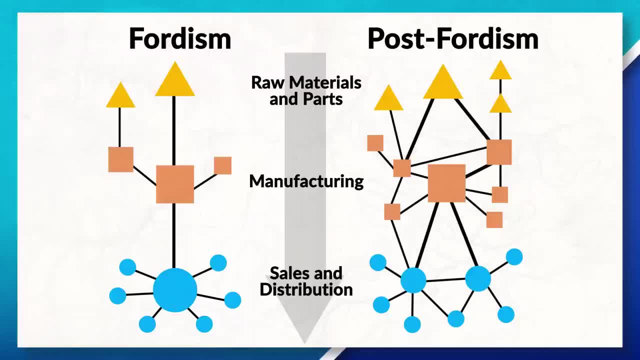 tasks and roles to allow for a more adaptable workforce. There is often less of a focus on standard goods and more of a focus on custom goods that meet the specific customer needs and wants. Post-Fordism also tends to use local decisions when it comes to production with production. 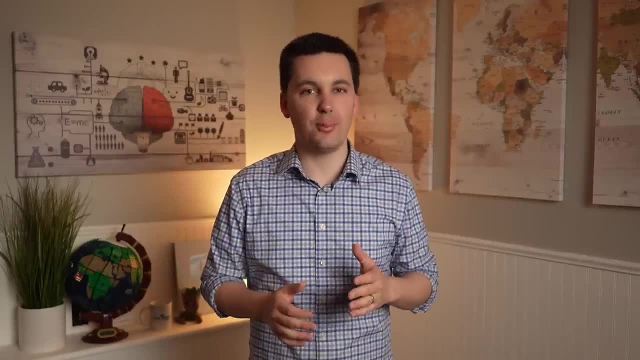 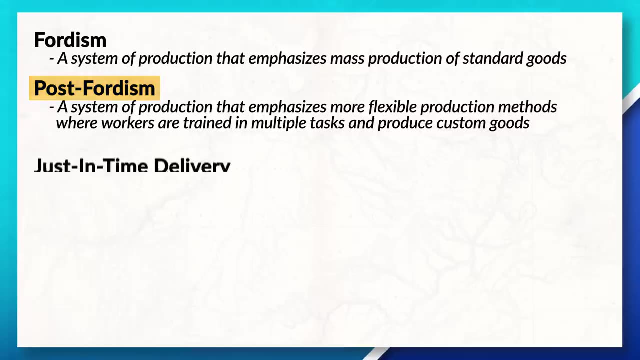 often being decentralized, meaning that production here no longer happens all in one location. Instead, goods are often produced in a variety of stages and locations. One way this is done is by utilizing a concept known as just-in-time delivery. This is when materials parts 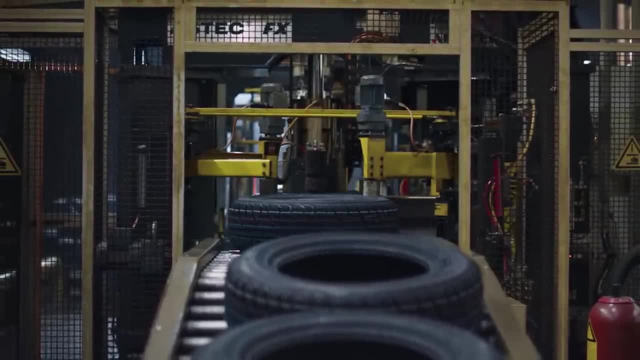 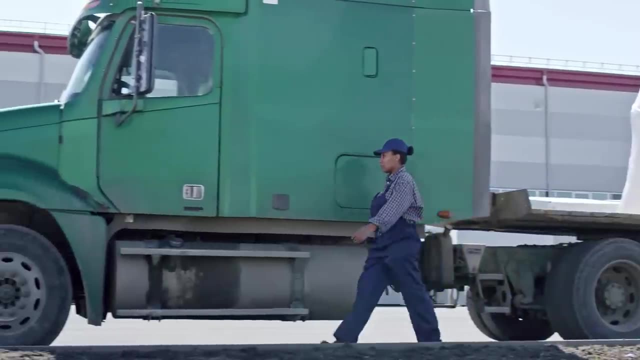 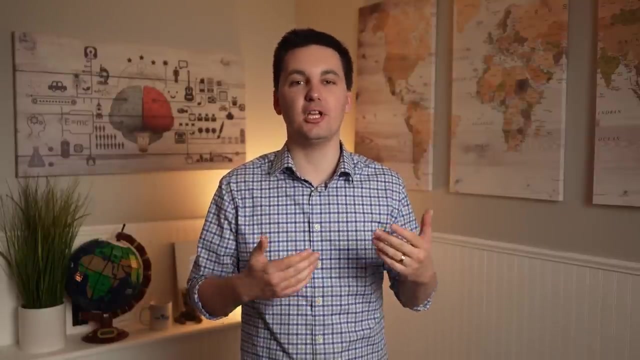 or products are delivered to a manufacturing facility precisely when they are needed. This helps reduce costs and waste by only having products arrive at the production facility when they are needed and only sending the exact parts that are actually going to be used for production. Just-in-time delivery helps reduce the cost of carrying inventory and increases the 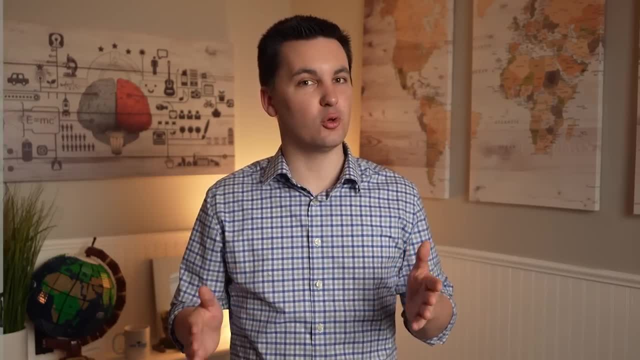 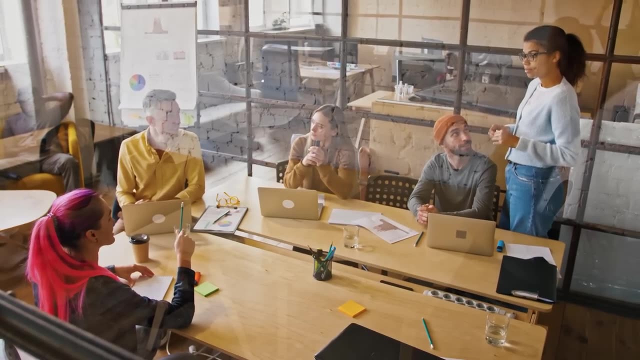 production capacity, But it also has some big risks associated with it. Any delays in the supply chains or disruptions can delay the entire production process. Also, just-in-time delivery requires a high degree of coordination between the different suppliers and manufacturers. If there is any miscommunication, 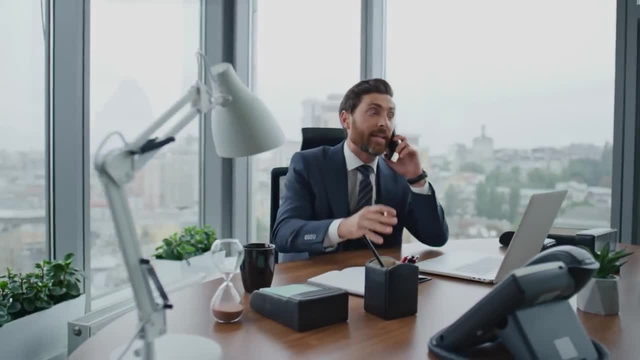 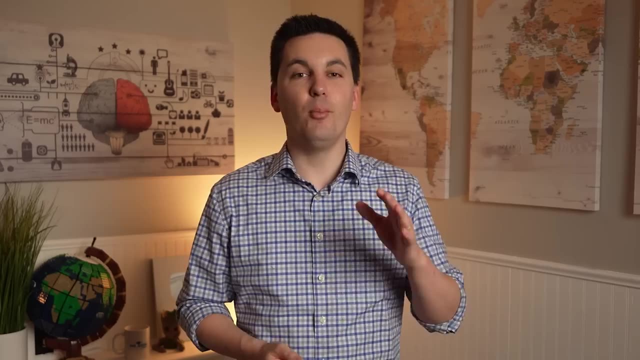 between the two, it could stall production and result in a loss of revenue. Now, as time goes on, we continue to see less companies and countries utilize Fordism when it comes to production and more companies start to take advantage of post-Fordist methods. 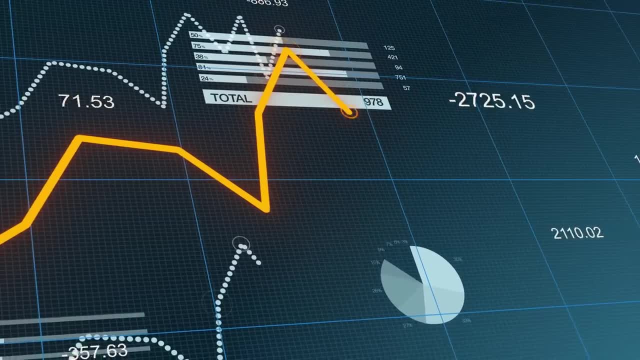 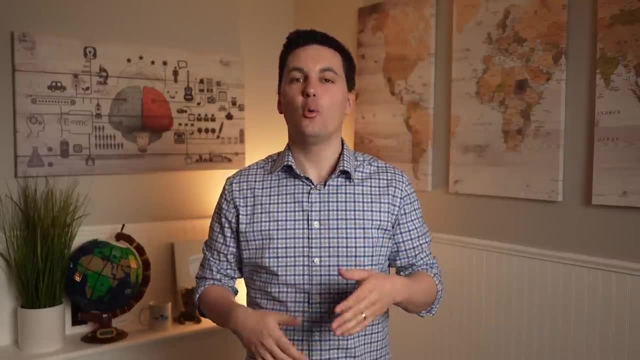 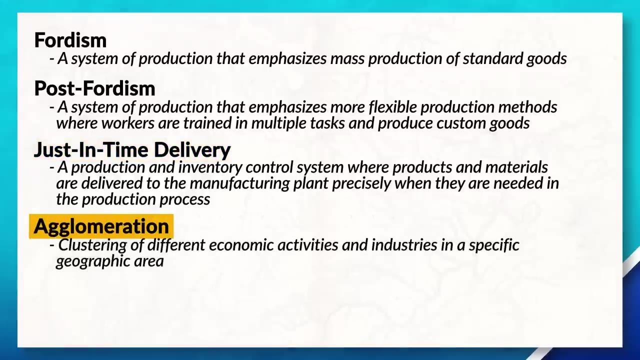 All of this is due to the changing market demands, technological innovations and increased globalization. Now, since we're talking about how production is now occurring in multiple stages and locations, we also need to look at the economic benefits of agglomeration and growth poles. Agglomeration is the clustering of different economic activities and industries. 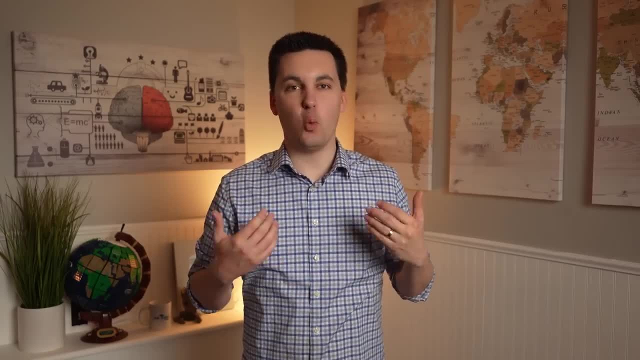 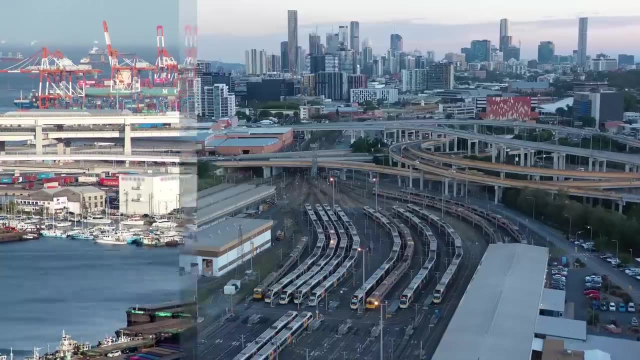 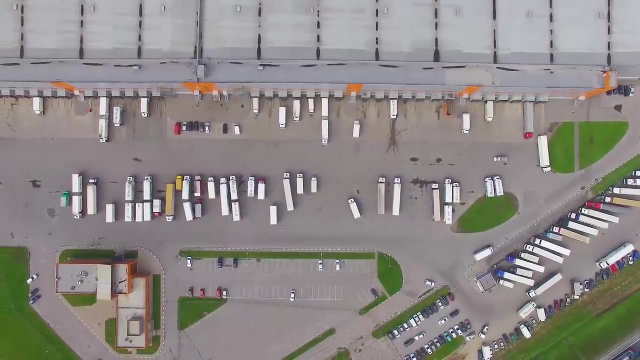 in a specific geographic area. This happens because businesses want to reduce their overall costs by taking advantage of a larger labor force benefiting from existing infrastructure in an area, utilizing different services and knowledge bases in an area. For example, we can see that many distribution centers will locate near major interstates, airports, rail yards and ports. This 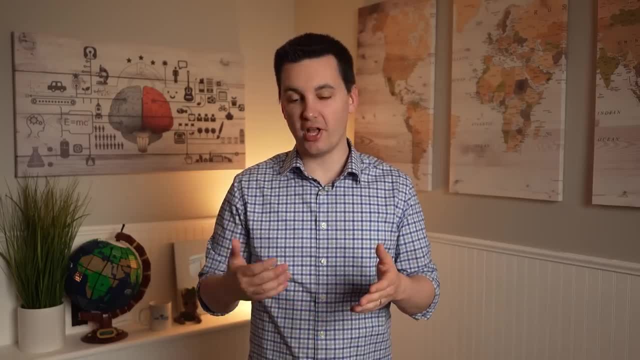 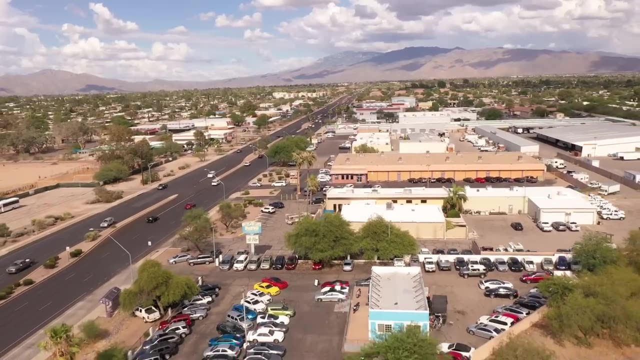 allows them to use the pre-existing infrastructure in the area instead of building it for themselves, which reduces the overall costs of their production. Traditionally, agglomeration occurs naturally, since it's in the company's best interest to locate in the area in order to help. 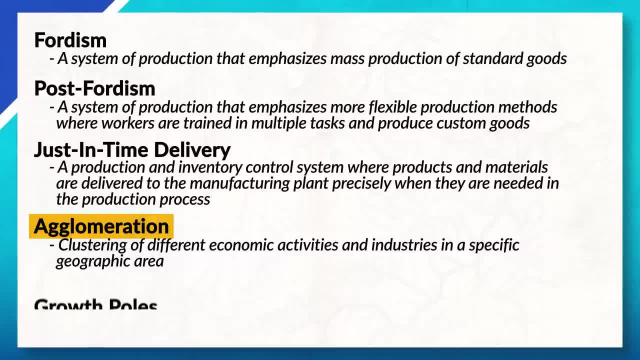 decrease their overall costs and increase their profits. Growth poles, on the other hand, are areas- cities- that are centers of economic growth. They're often created by either targeted public or private investments. We can see that targeted investment can be done in a variety of different 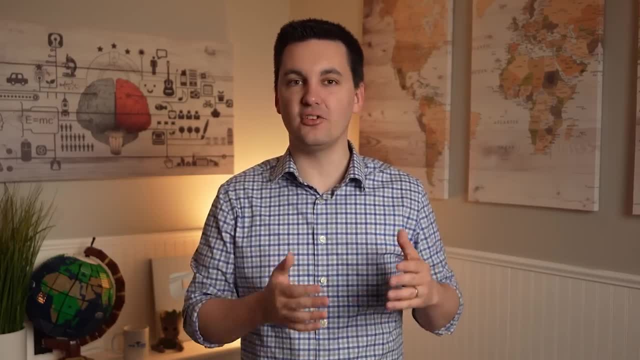 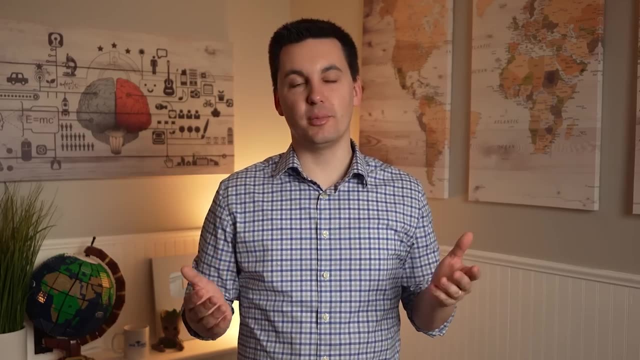 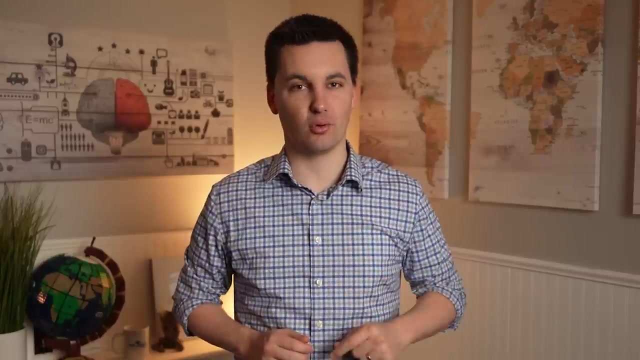 ways, such as by creating specific infrastructure that meets the needs of the businesses in the area, For example, creating more transportation routes or energy for companies in the city. We could also see governments create specific policies and investments in an area which create a pro-business environment for economic growth, For example, Silicon Valley in California.